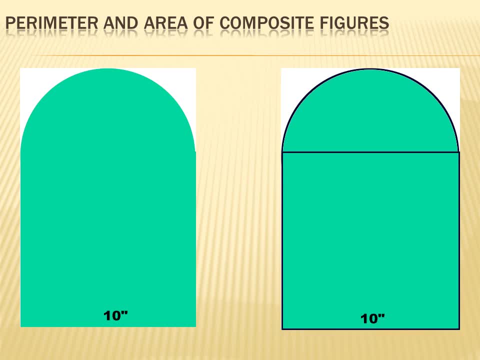 plus this distance, plus this distance, the distance around the shape. It wouldn't include this line because this line's not around the shape, it's within the shape. So the perimeter would be that side plus that side, plus that side, all of which are 10 inches. 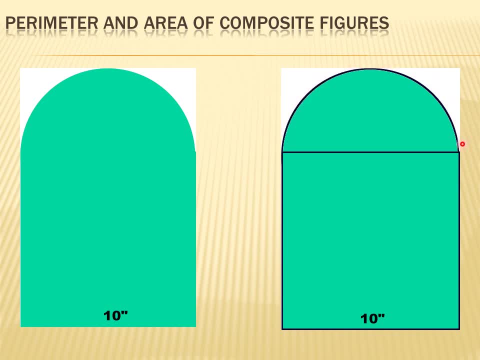 plus one-half of the circumference of the circle, that would complete this semicircle. Let's figure that out. The perimeter of the semicircle is one-half pi d, or one-half times 3.14 times 10, which equals 15.7 inches. 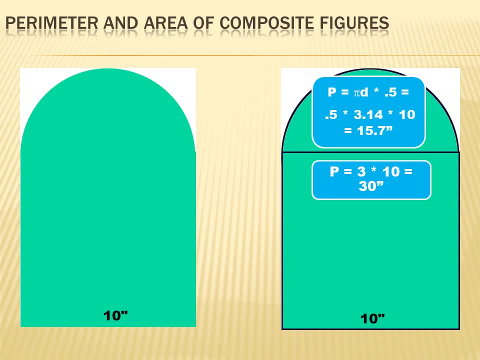 The perimeter of three sides of the square is 3 times 10,. 3 times 10 inches, or 30 inches, And the perimeter of the entire shape, the entire composite figure, is 15.7 plus 30 inches equals 45.7 inches. 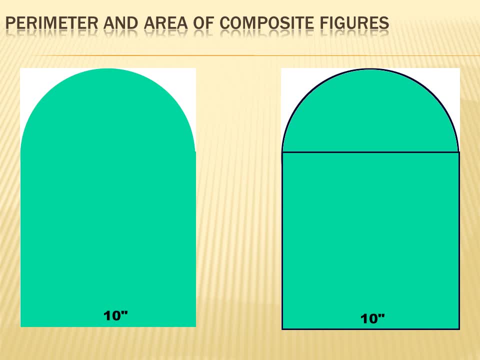 Well, how about the area of this composite figure? Hopefully you can see that the area is made up of the area of the square, the 10 by 10, plus the area of the semicircle, And the area of the semicircle would be half the area of the circle that completed the semicircle. 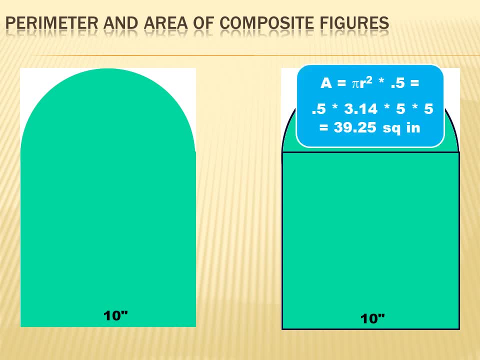 So let's calculate the semicircle first. The area would be the area of the entire circle, pi r squared times 0.5, since we've only got half a circle. So to calculate it, we calculate 0.5, or half times pi. 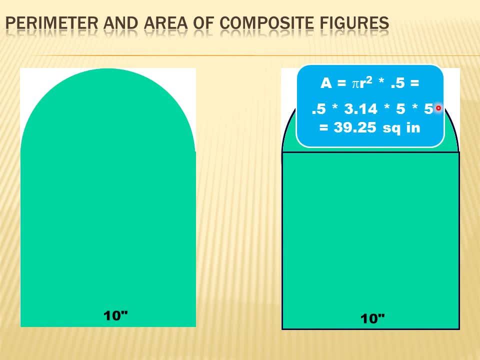 times the radius 5 inches. squared, The radius is 5 inches because the diameter is 10 inches and the radius is half the diameter. 0.5 times 3.14 times 5 times 5 equals 39.25 square inches. 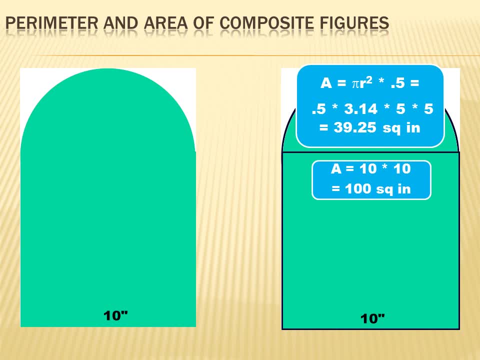 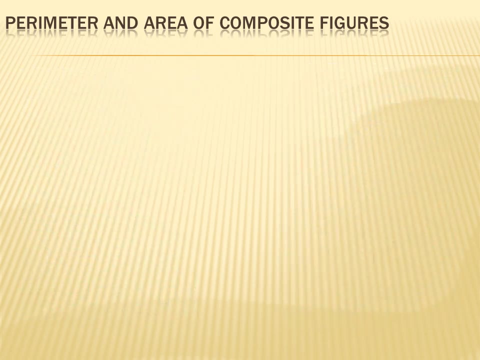 Now the easy part. The square is 10 by 10, so the area is 100 square inches And the combined area would be 139.25 square inches. Well, you can see, you need to know some math to do these problems. 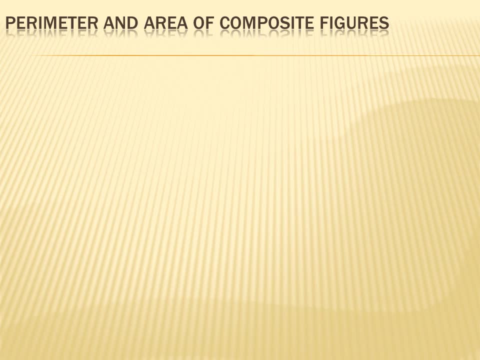 You need to be able to calculate the perimeter and calculate the area of rectangles and squares and circles, but I think you can do that. The other thing you have to be able to do on this is really the puzzle-solving portion. It's to look at the figure and use your brain and try to figure out. 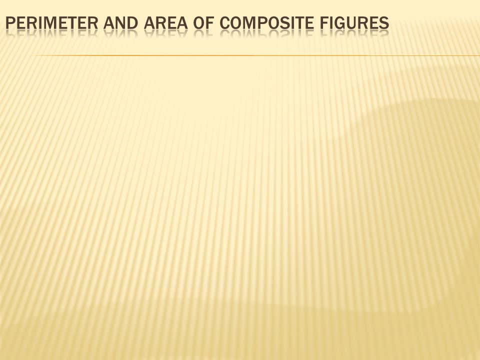 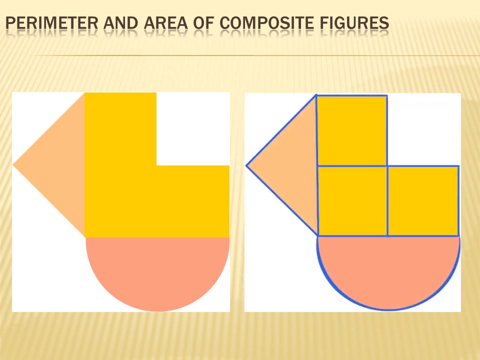 what individual shapes were pushed together to compose this figure. Let's say we had a figure that looked like that. That's a pretty strange-looking figure, But I think you can see it's really several figures pushed together. We have a triangle, We have three squares. 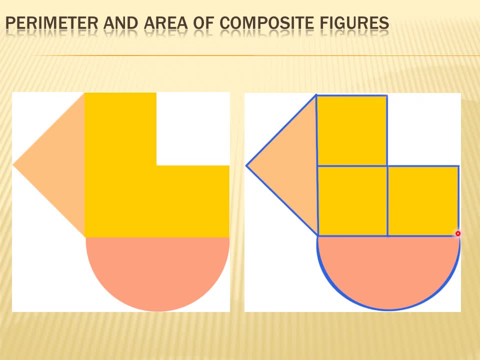 Or we have three quarters of a larger square. Either one is correct And we have a semicircle. So if we knew enough dimensions, we could figure out the area and the perimeter of this strange shape. Try this one. Hit the pause button. 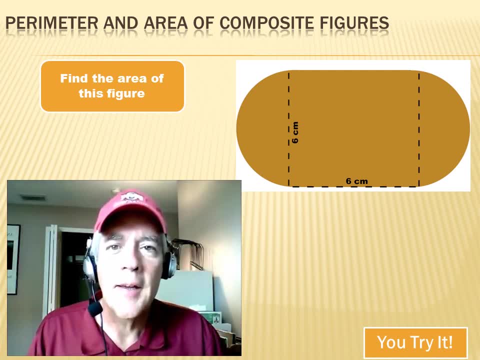 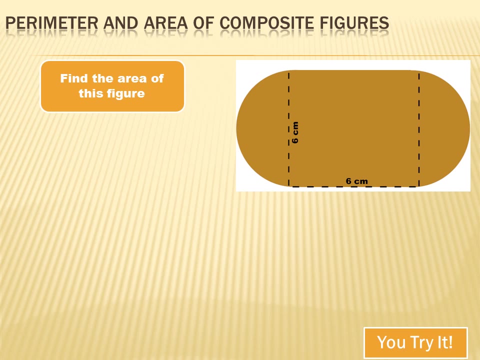 do the problem and then hit your forward key. Well, if we need to figure out the area of this figure, we need to figure out what the composite figures that make up this figure are. So let's look at it. I see a square that's six centimeters by six centimeters. 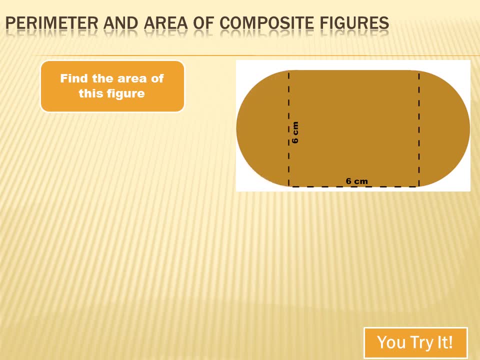 And then I see a semicircle over here that has a diameter of six centimeters, And I've got an identical semicircle over here, which would also have a diameter of six centimeters, So I've got two semicircles. 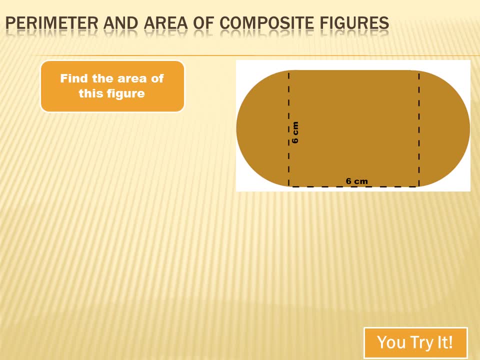 which is equal to one circle plus. I've got one square, So let's first figure out the area of the circle. The formula is pi r squared, So that's 3.14 times the radius squared. The diameter is six centimeters. 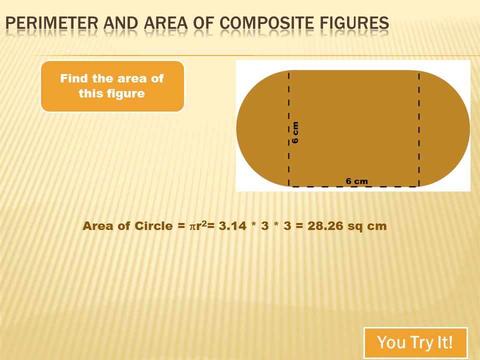 so the radius is three centimeters. So 3.14 times three times three equals 28.26 square centimeters. Now I need the area of the square. The square is six centimeters by six centimeters, so the area is 36 square centimeters. 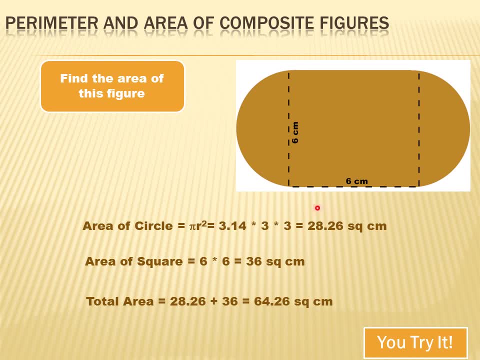 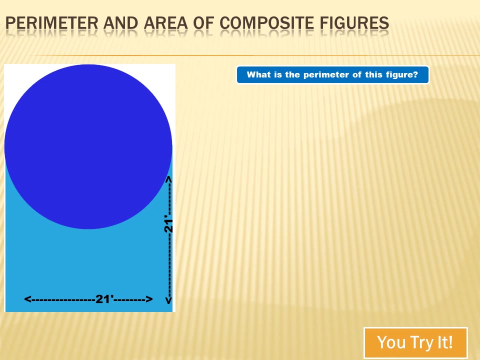 And the total area of the composite shape is the area of the semicircles plus the area of the square. 28.26 plus 36, equals 64.26 square centimeters. Well, in order to figure out the perimeter of this figure, 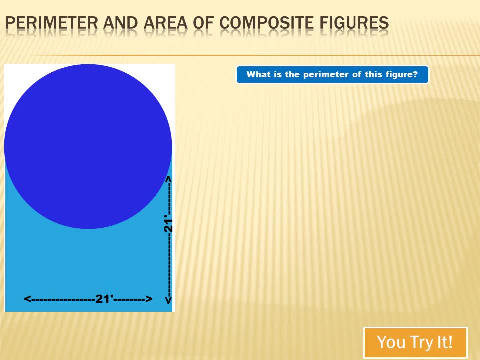 I need to understand what shapes compose this figure. what shapes were brought together to make up this figure? And I can see that there's a circle on the top And I can see that it's sitting on what appears to be a square. So the perimeter would be the distance. 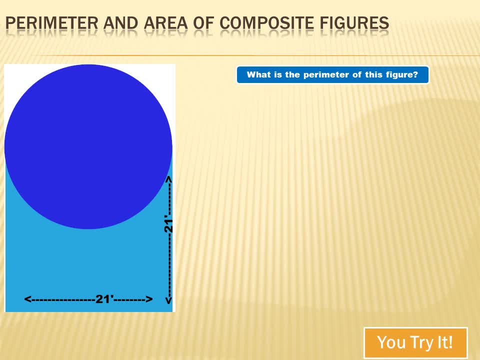 all the way around the outside of the composite figure And that would be made up of half of the circumference of this circle plus this side, this side and this side of the square. Half the circumference of the circle would equal 0.5 pi d. 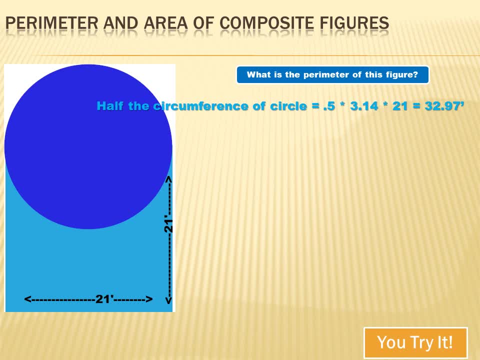 or 0.5 times 3.14 times 21, or 32.97 feet. Three sides of the square would equal 21 feet plus 21 feet plus 21 feet or 63 feet, And when I total those two dimensions together, 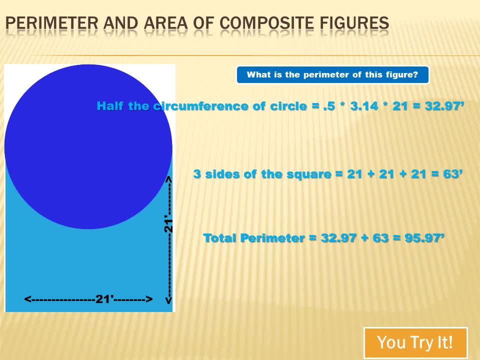 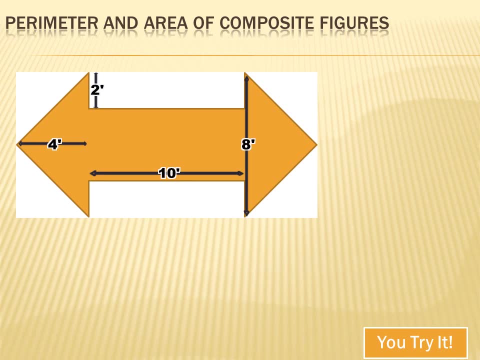 I get 95, 95.97 feet. The trick to figuring out the area of this composite figure is to break it up into its components and figure out what the area of each of those are. I can see a triangle here. I can see an identical triangle over here. 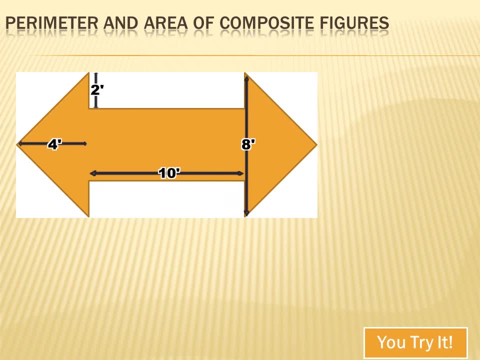 And I can see a rectangle between them. Well, let's figure out the area of each of those triangles first. The formula for the area is one-half the base times the height, So I plug in one-half or 0.5.. 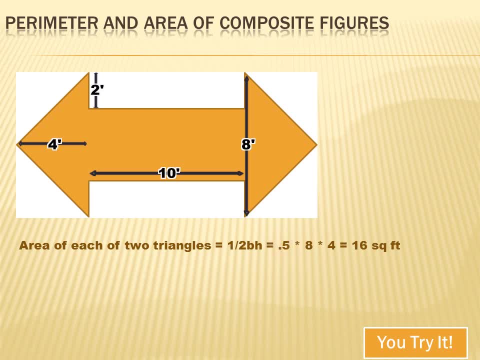 I plug in the base, which is 8.. I know it's 8 because these are identical and that's 8, so both of them are 8.. And then I plug in the h, the height, which is 4.. 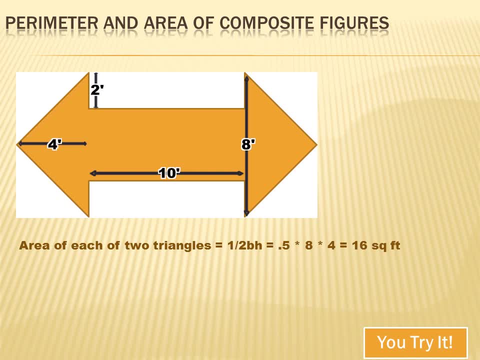 0.5 times 8 times 4 is 16 square feet. Now you've got to remember that's the area of each of the triangles and I'm going to have to double that when I combine them with the rectangle for the total area. 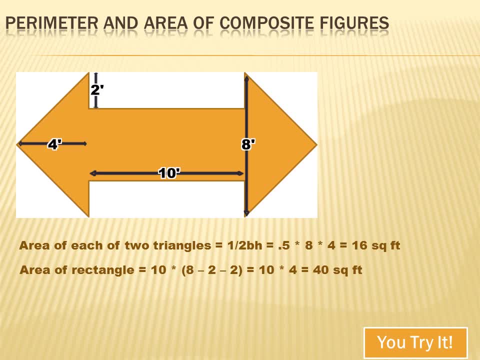 Now let's figure the area of the rectangle. The area of the rectangle is the base times the height. But they don't give me the height. They give me that dimension which is 8 feet, And they give me that dimension which is 2 feet. 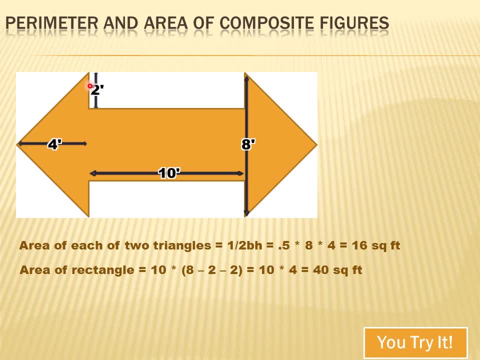 And I can assume that this dimension is the same as that dimension, And I can assume that this dimension is the same as that dimension, And I can assume that this dimension is the same as that dimension. So this is also 2 feet, But they don't give me this dimension. 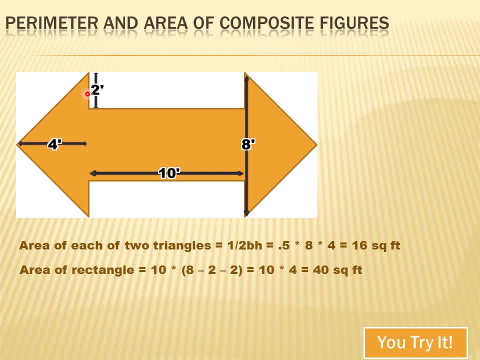 Ah, but fortunately I'm smart and I can figure that out. That's 8 feet, but I'm taking away 2 feet here and another 2 feet there. So 8 minus 2 minus 2 is 4.. 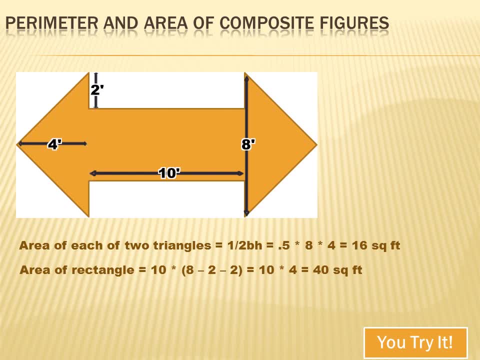 And my rectangle has a height of 4.. So to calculate the area of the rectangle, So to calculate the area of the rectangle, I multiply 10 times 8 minus 2 minus 2, and that equals 40 square feet. 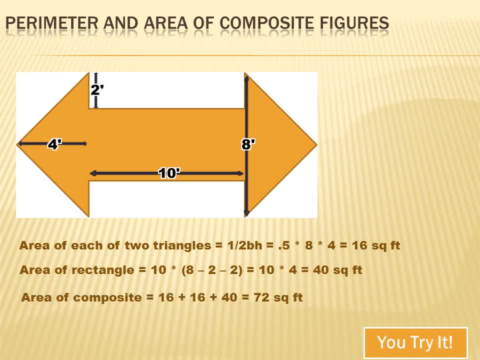 Now the composite figure is the sum of 2 triangles, each 16, so I get 16 plus 16, plus the area of the rectangle at 40, where our total is 72 square feet plus the area of the rectangle at 40,.